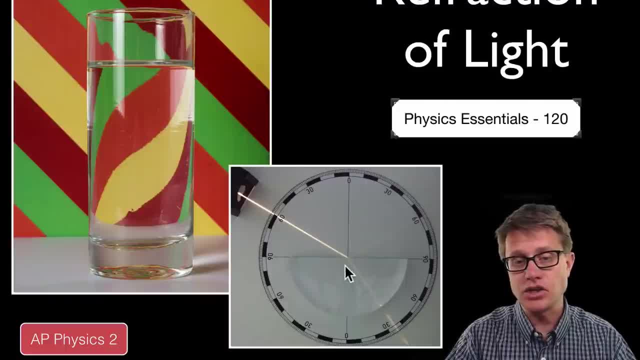 light like this, And the reason it is bending is because we are changing the speed at which it is moving through the medium, And I will give you an analogy that is going to help you in a little bit: What would happen if we go straight into the medium. It is just. 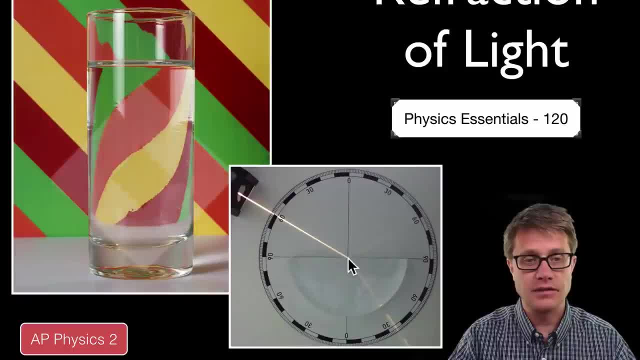 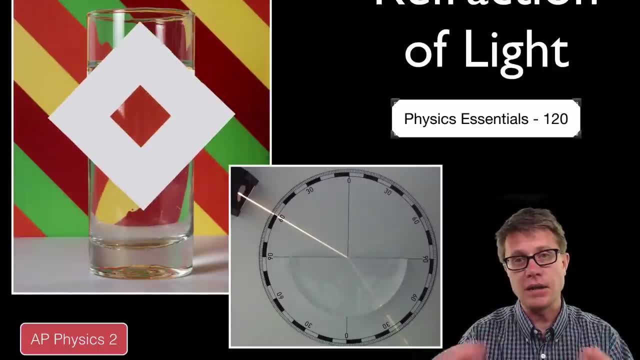 going to go straight through, And so if you look on the glass to the left, the light that is coming straight through the middle, where the surface is flat, it is not being refracted at all. It is only on that bent surface where we see. 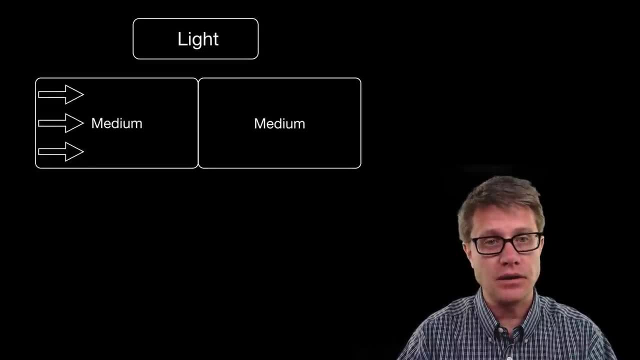 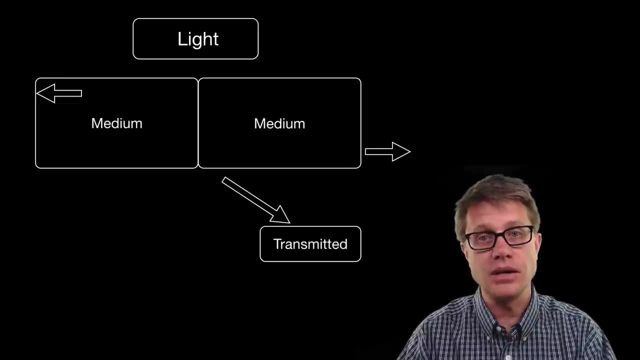 that major refraction, And so when light moves from one medium to another, it can be reflected, absorbed or transmitted. Now, in this video, we are dealing with light that is transmitted into that other medium. Now, in this example, however, the light came in. 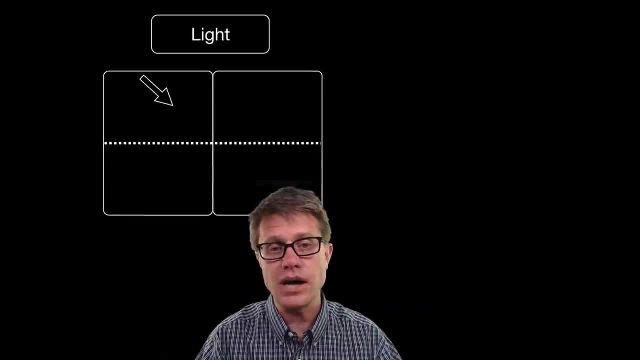 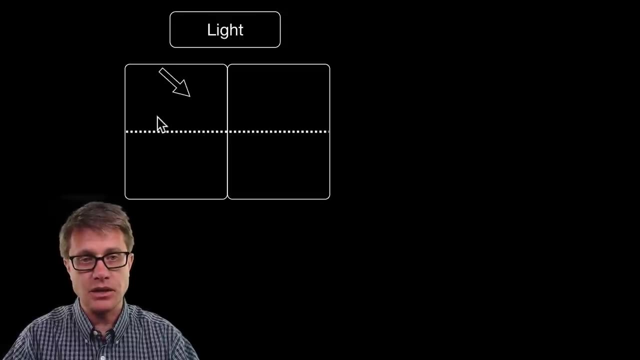 at a straight angle, And so we do not see that refraction. But what happens if it comes in at an angle that is not along the normal or not along the perpendicular? And so these are the two mediums, This is the one on the left and the one on the right. This would 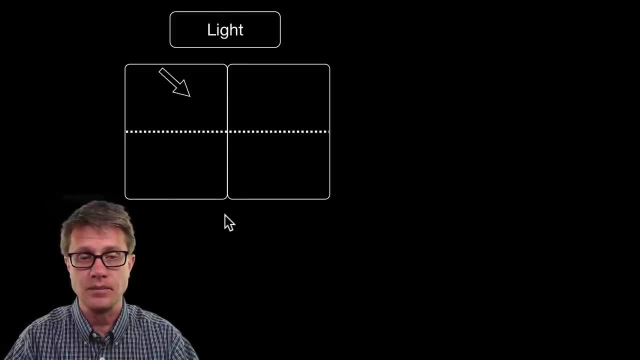 be the boundary between the two, And then this is the normal line right here. So this here. And so what happens? if it comes in from one medium, enters another medium where it is going the same exact speed. there is going to be no change in the angle, It is just going. 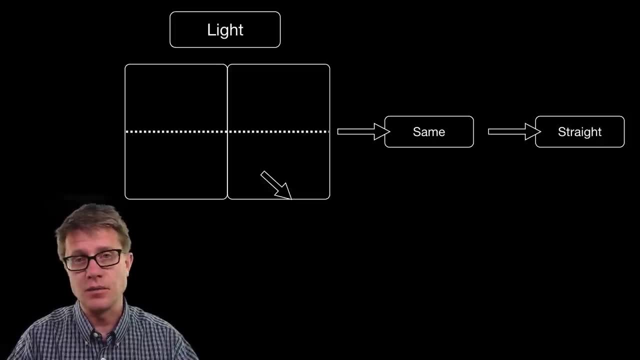 to go straight through, Just like light goes straight in air, because the medium is never changing. What happens, however? if it goes from one medium to another and that second medium it actually travels slower, As it does that it will actually bend towards the normal, or it is going to bend towards that dotted line or the perpendicular line I will give. 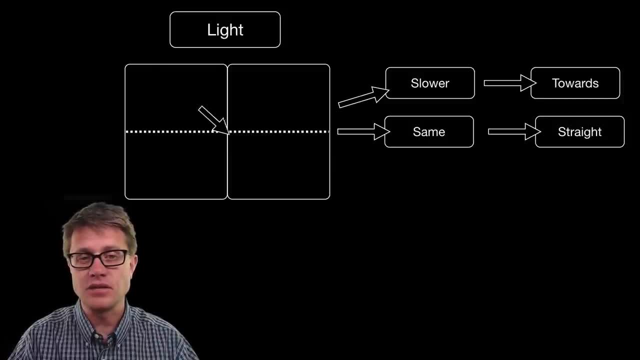 you an analogy that will help you to remember that. What happens if it comes in and it is moving into a faster medium? It will actually bend away from that normal. So it is going to bend like that. Now that is called refraction, where you see the bending of the light And 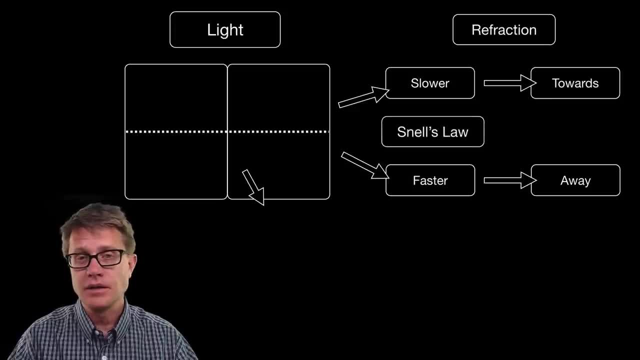 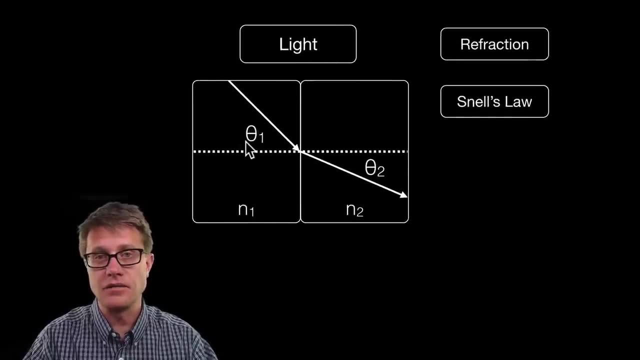 we can actually quantify that using something called Snell's law. Snell's law. to quantify it, we have to add a couple of different variables. We first of all have to define this as the angle of incidence And this as the angle of refraction. Again, we are always measuring the angle between. 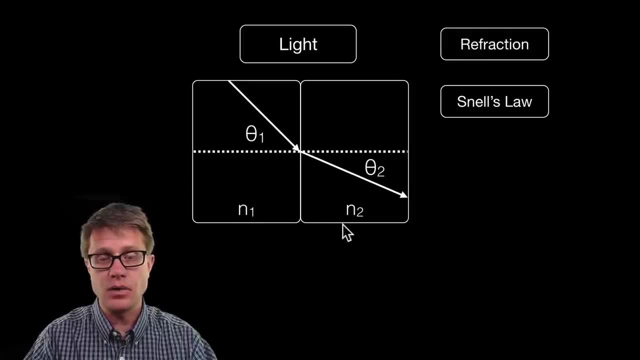 the normal and the light ray itself, And then we have n1 and n2.. So this is what the formula for Snell's law looks like, And so the index of refraction- we call that n1, on one side times the sine of the angle equals the index of refraction on the other side times the 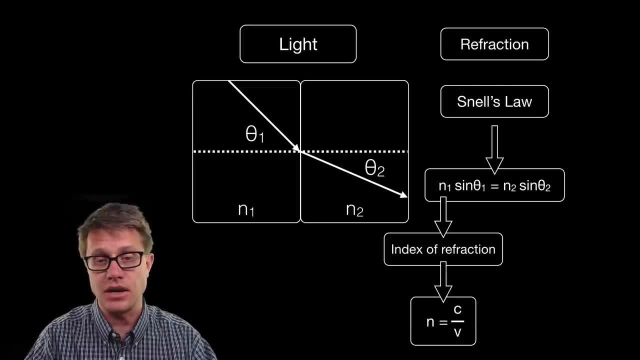 sine of the angle, angle of refraction on the other side, And so we can actually figure out what angle it is going to bend at. if we know a little bit about the speed at which it is going through And we also if we see the bend, we could figure out the speed at. 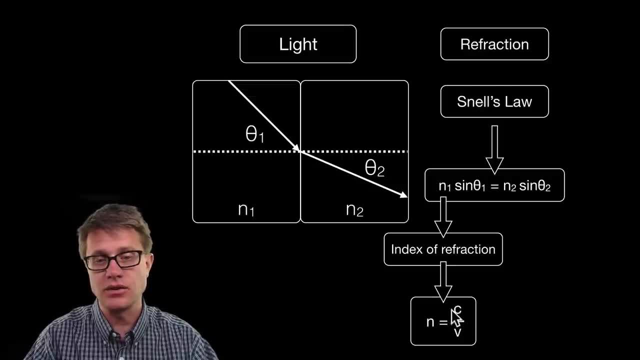 which it is going through as well, Because the index of refraction is equal to the speed of light divided by the velocity. Now if we take that angle and we start to increase it, increase the angle of incidence- we eventually can reach what is called a critical angle. 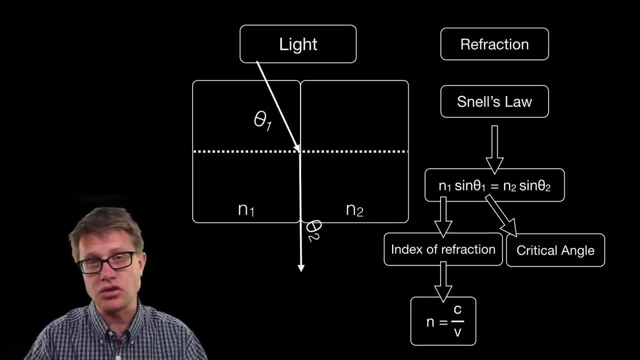 And instead of being refracted, it will not be refracted, it will just go straight along the margin. And if we increase it above the critical angle, then it is going to be reflected into that first medium. And so what happens is, eventually, if you get the angle right, you 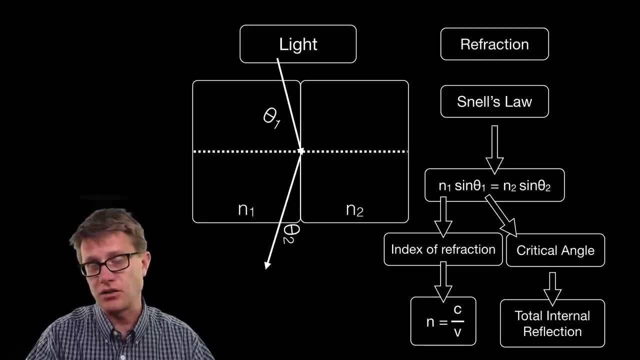 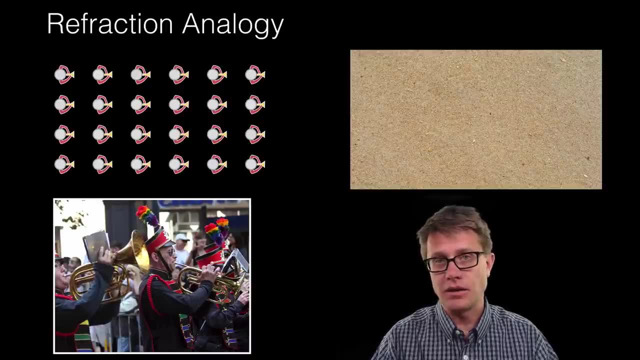 will have total internal reflection. None of it is being refracted or transmitted through that boundary. And so let's get to that analogy I was talking about a second ago. And so imagine we have a marching band that is all walking together, And so we are looking at the marching. 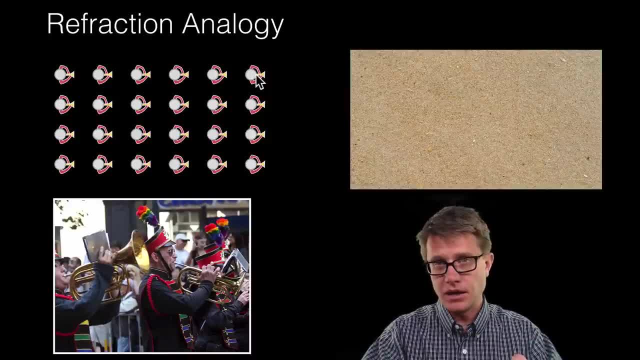 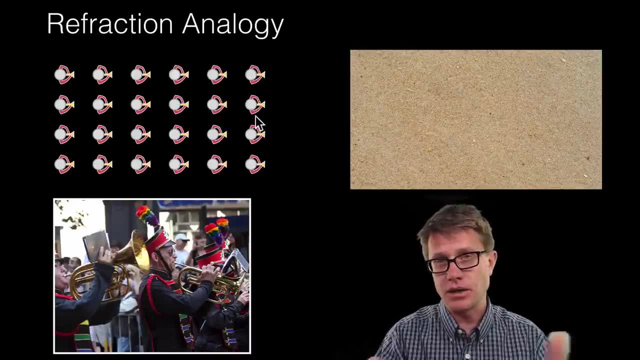 band, the trumpet players, and we are looking at them from above And as they are marching, they are trying to keep the space between them the same. So, to the person to your left or the person to your right, we want to keep that exactly the same, And so imagine that. 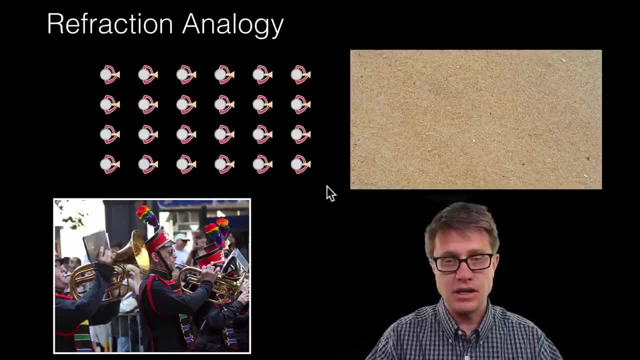 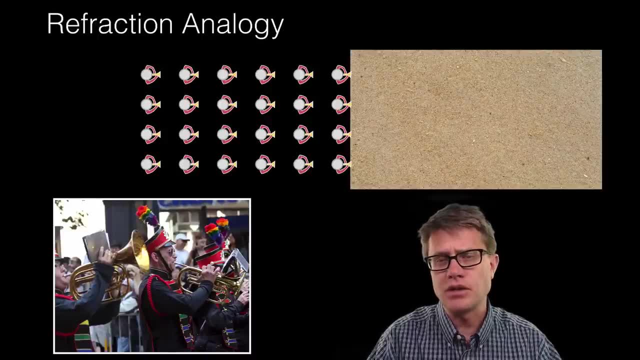 they are marching down a road, You can see that they are going to keep that spacing between them the same. But let's say that there is a bunch of sand in the road, And so what is going to happen to their speed as they enter into the sand? Well, the ones that enter into. 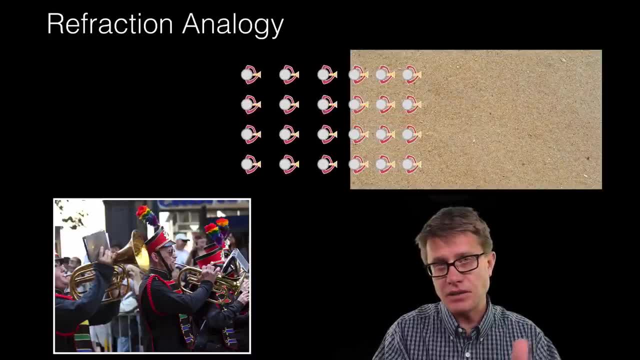 the sand first, are going to slow down. But since they kept that distance between them the same, you can see that the 0 angle at which we came in equals the angle at which we came out. So we do not see that refraction going on. But now let's set it up so they are marching in at an angle like: 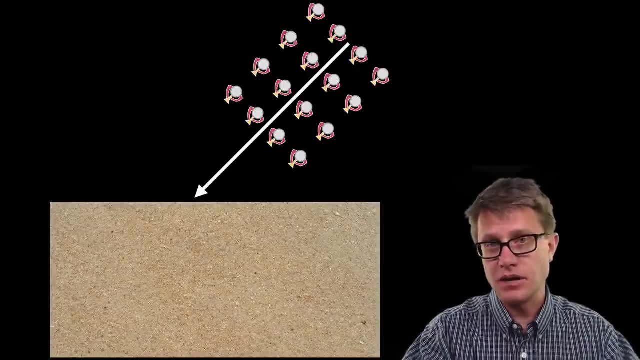 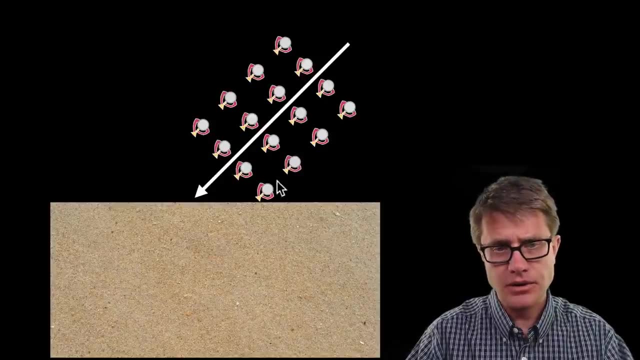 this, And so they are marching across, let's say, a parking lot, And they are going to hit some sand as well. So what happens is, as they come in, which one is going to start to slow down first? Well, it is going to be this one right here. They are still going to keep this. 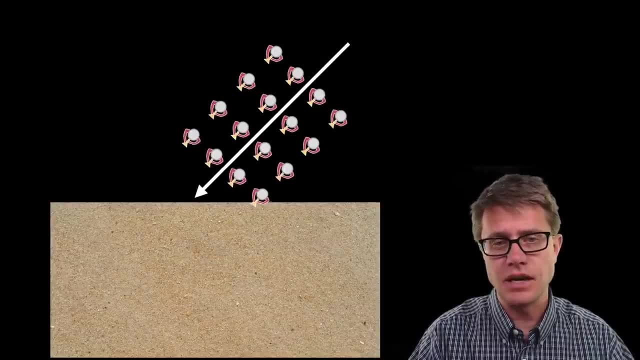 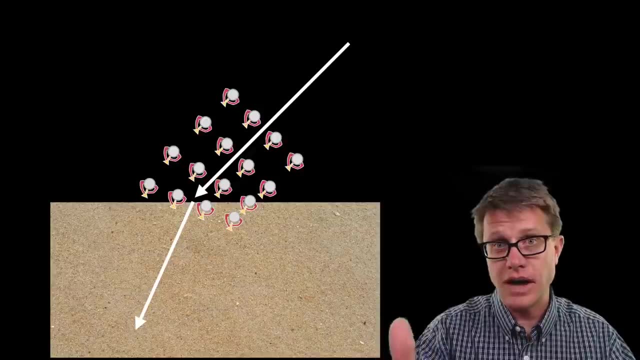 distance between all of them the same, And so watch what happens as they enter into the sand. You can see they are bending like that, And so we are going from a medium where it is faster, to one where it is slower. So if I put in that normal right here what happened, 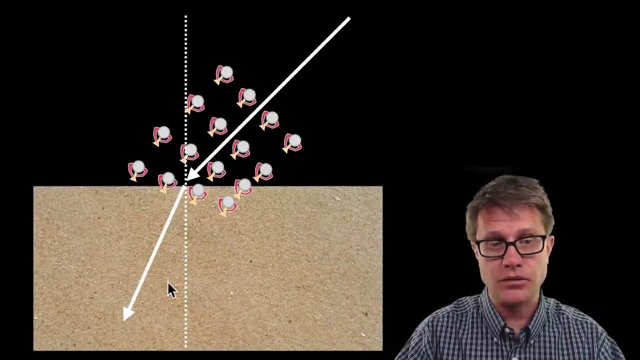 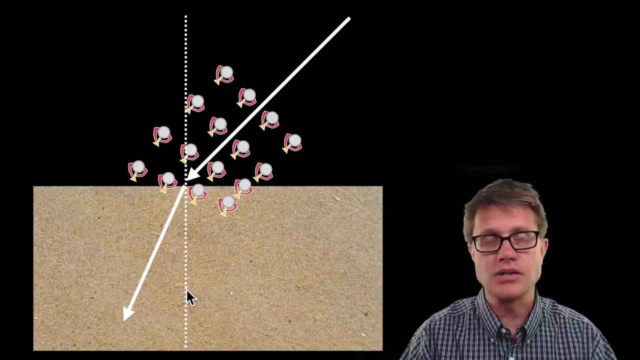 This is our angle of incidence, So it is big. What happens to our angle of refraction? It is going to be small. In other words, it is approaching that normal, And so you always, when you are looking at problems with refraction, you want to imagine that marching band in. 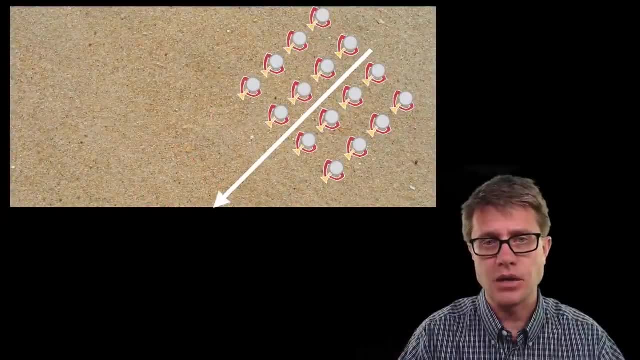 your head and figure out which way it is going to go. So let's try that again. We have got a marching band now going through sand And they are going to hit some sand And they are going to come out into an area where they go faster. So they are all going slow, but 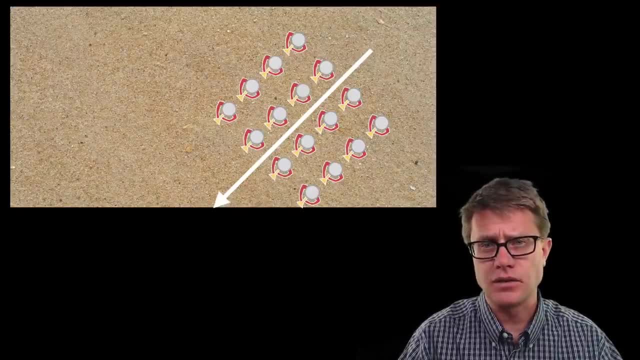 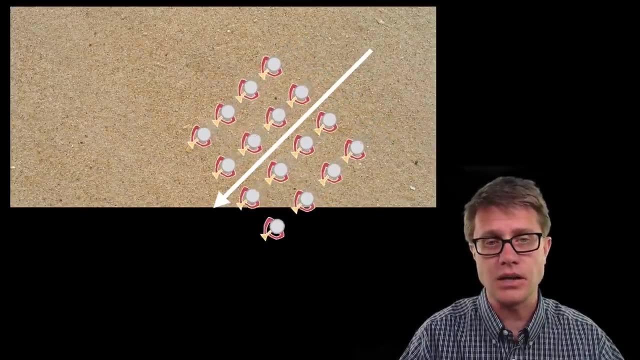 they are going in a straight line. Now which one is going to start to go faster first? Well, it is going to be this one right here. They are keeping the distance between them all the same, And so watch what happens now. So it is bending like that, And so if we put 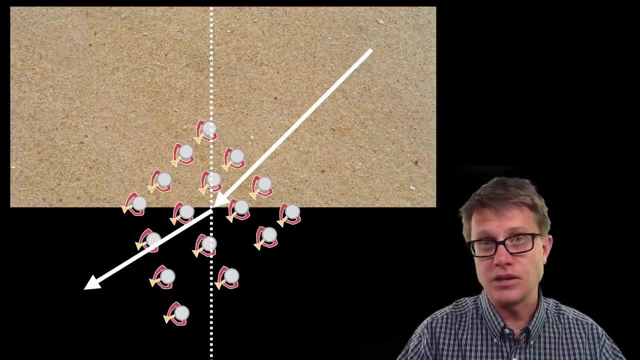 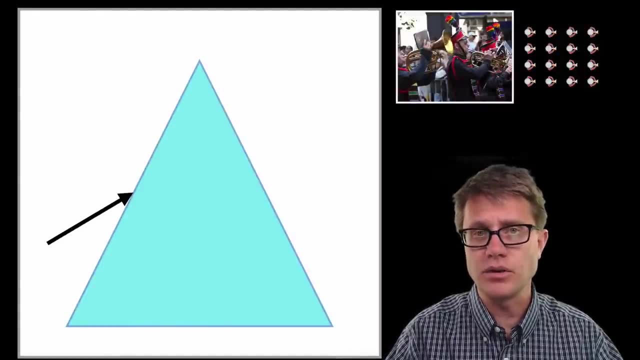 in that normal again, our angle is actually increasing. Our angle of refraction is going to be bigger. Let's try to apply that with a prism. Let's say that we have a light ray coming into a prism. We are going to have a light ray coming into a prism. We are going. 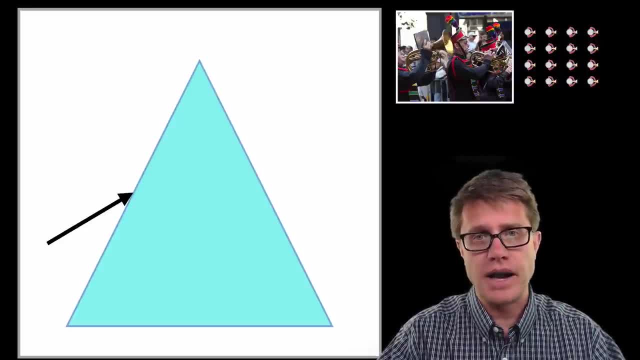 to have a prism like this, And inside the prism the light goes slower, So in the glass it is going to go at a slower rate. And so what is going to happen as the marching band approaches? try to figure this out in your head. I can see that the right side is going. 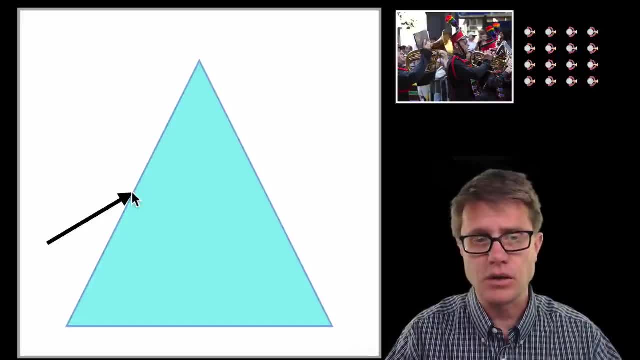 to start to slow down first, And so if that does not work, you could just memorize, Put in the normal and then figure out what happens to our angle of incidence and angle of refraction. But it is going to bend to the right like that. What happens if we go to the next one? 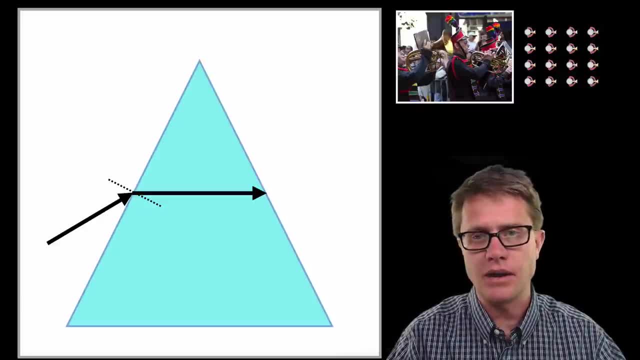 So which side of the marching band is going to start to exceed the normal? Well, the right side of the marching band is going to start to accelerate first as we move out. It is going to be the left side. If that does not work, again, you could put in the normal and 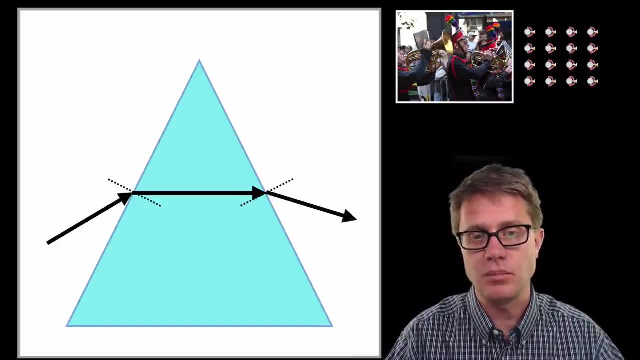 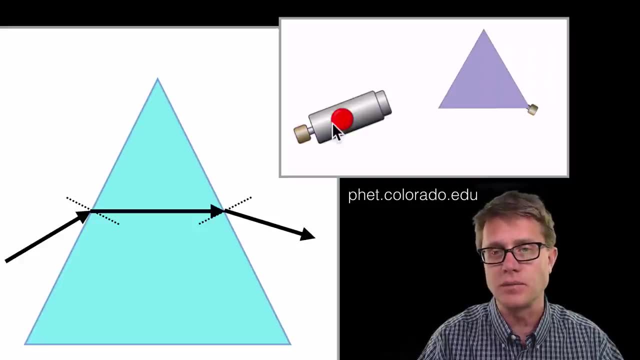 we could say that we are going to see an increase in that angle of refraction, or it is going to bend like that. Now we could even make sure that that is right, And so this is a PHET simulation. You can shoot a laser at different prisms. So if I turn the laser light, 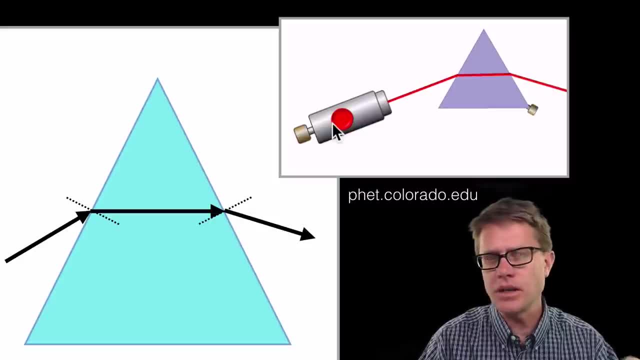 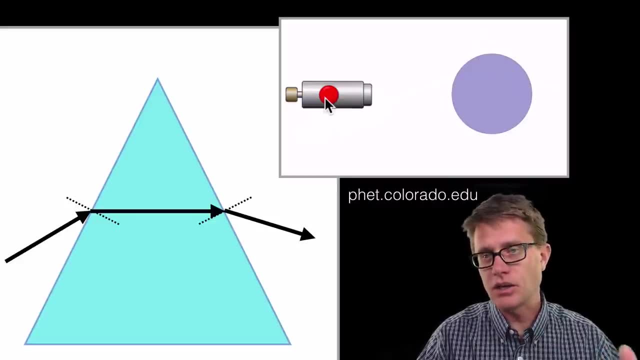 on, we can see that refraction occurring, And once you figure out this analogy, it works really well. So, in other words, what is going to happen if we shine a light right at a sphere and we are going to try to hit it right along the normal, So it is hitting it flat? What? 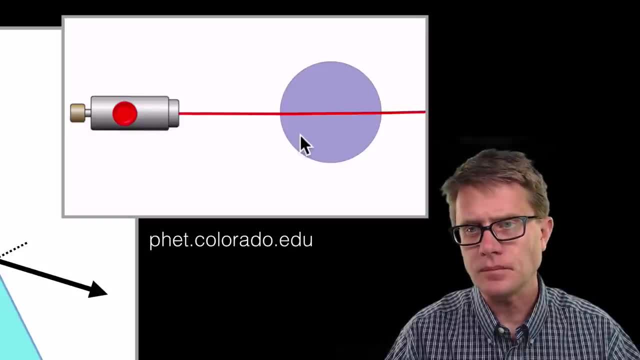 should happen to the refraction. Let us try it. You can see it is not lined up perfectly, but it is going to go straight through. Let us try another one. What is going to happen here if we hit it at an angle like this, Where is going to be the bend, And so which one? 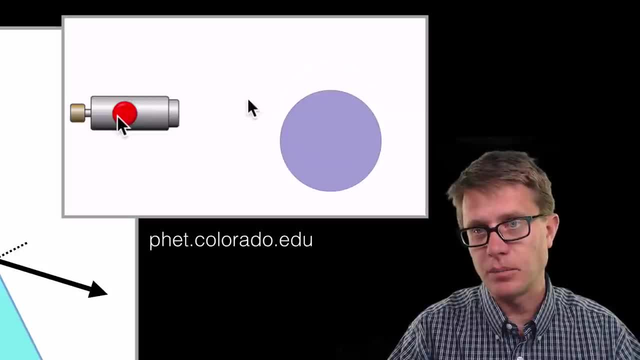 is going to start to slow down first. I would say the marching band. you know, put yourself in that position. but the marching band on the right side is going to slow up first. What is going to happen as we bend, as we come out here? Try to figure out what is going. 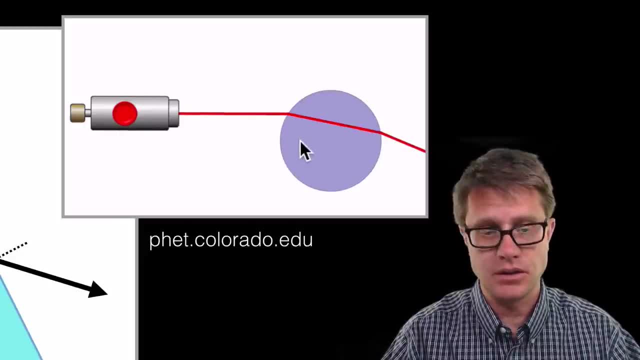 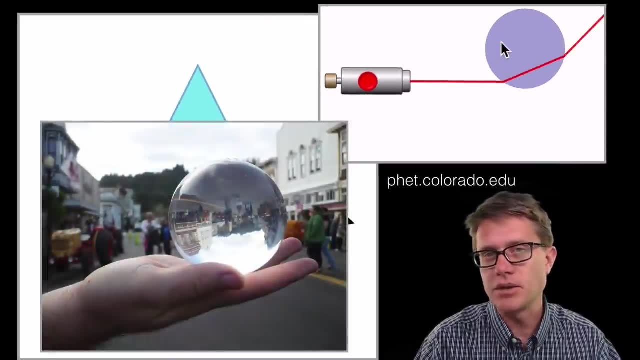 to happen in your head, But this is what it would look like. So we are going to get refraction that looks like that, And so you can see, the more I get that bend, the more refraction. Or I could go in the other direction. That is why we could hold this sphere up. 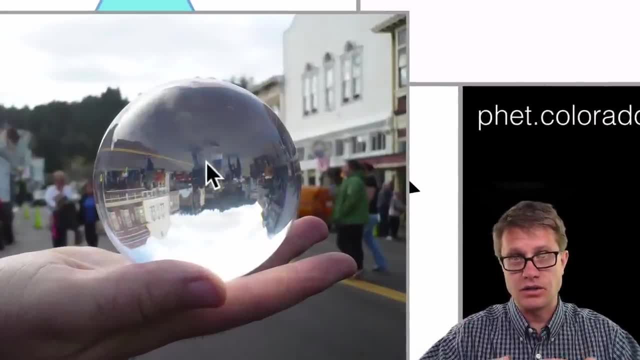 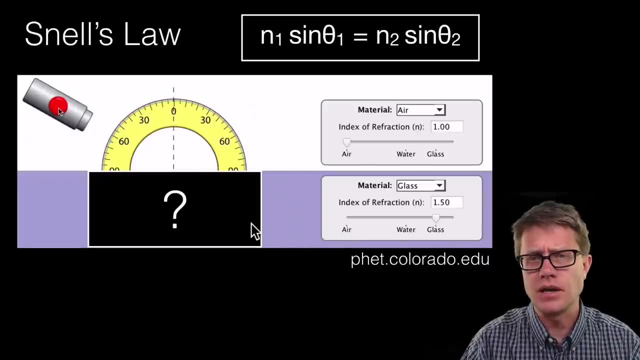 And if we look at it, the light coming from the other side is getting inverted. It is turning upside down due to the refraction of the light coming through. Now let us quantify a little bit. So we are going to use Snell's Law in a PHET simulation. Remember the index? 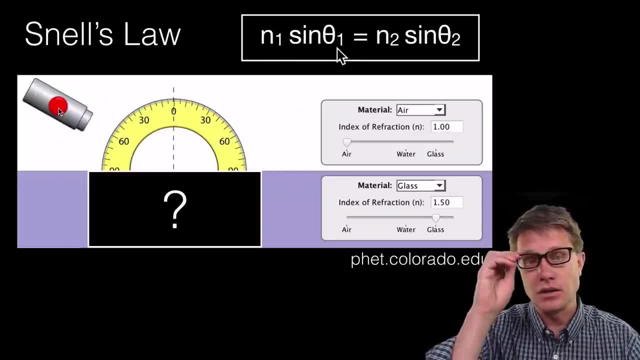 of refraction times, sine of the angle of incidence, how it comes in, Equals the index of refraction on the other side. And so index of refraction, remember, is related to the velocity, And so the index of refraction goes up as the velocity decreases. 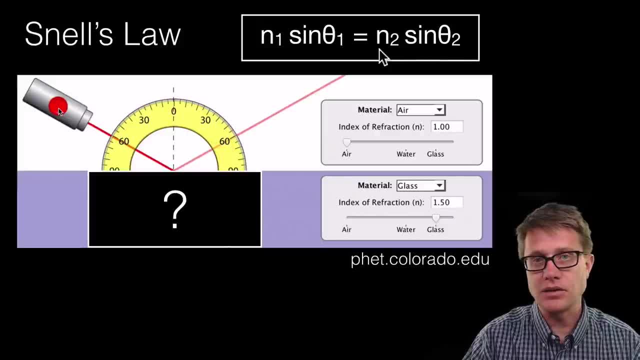 So let us take a look at this. So we have got a laser light bouncing off the surface And so you can see there is a lot of reflection going on, But a lot of that light is also going to be refracted on the surface. And so in this problem, if you know the angle at 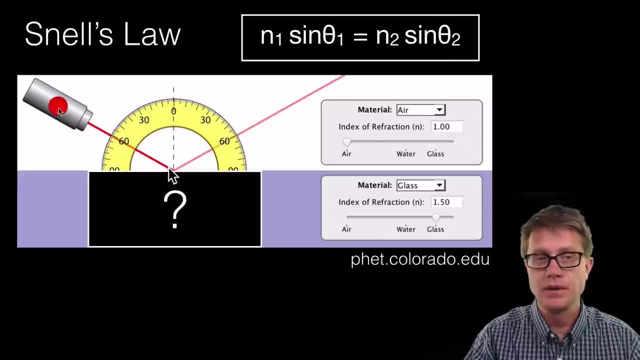 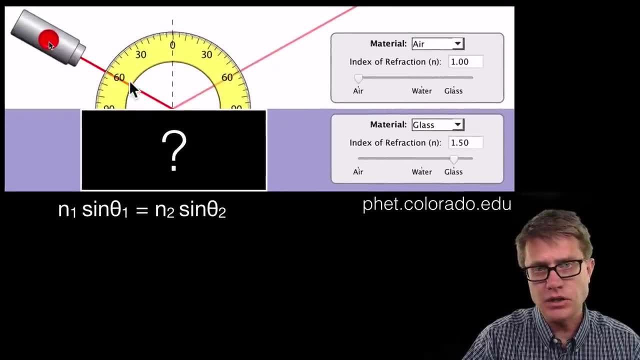 which it comes in. could you figure out the angle of refraction? you need Snell's Law to do that, And so I write it out like this, And then let me look at what information I have. So I have the angle at which it is coming. 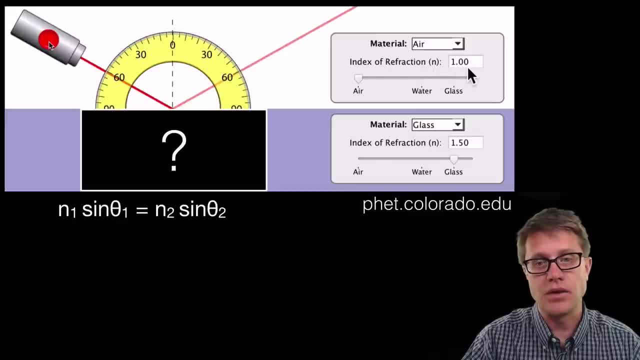 in. So that is a given. I also know. in air the index of refraction is 1.. I am also given the index of refraction of the surface down here, The glass is 1.5.. And so what? I am really? 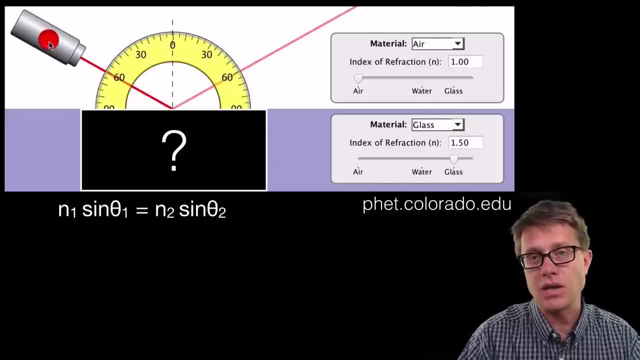 trying to solve, for I want to figure out that angle of refraction, How it comes out. So that is going to be my theta2.. So I plug in what I know. plug in what I know. So this is index of refraction of the light, The angle coming in, Index of 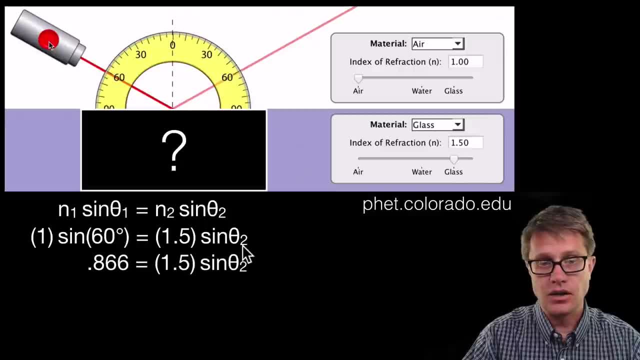 refraction of the glass And this is the angle coming out. So I solve for that. Now I have got sine of theta 2 equals 0.577. So I have to take the inverse sine to figure out what that angle is going to be. And so I get around 35 degrees, And so you may want to pause the. 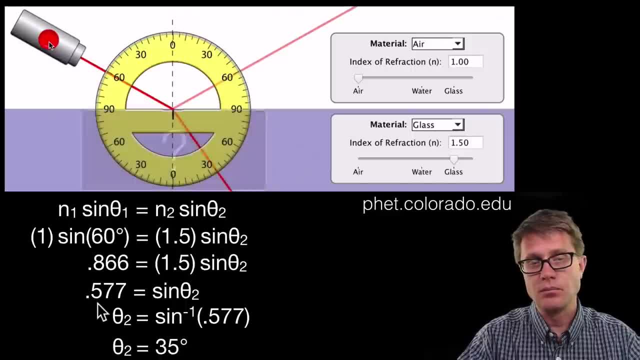 video and make sure that you get an answer that is similar to that, And now we could remove the question mark And you can see that that angle is going to be at 35 degrees. Also, you can see it is less, And the reason it is less is we are going from an area where 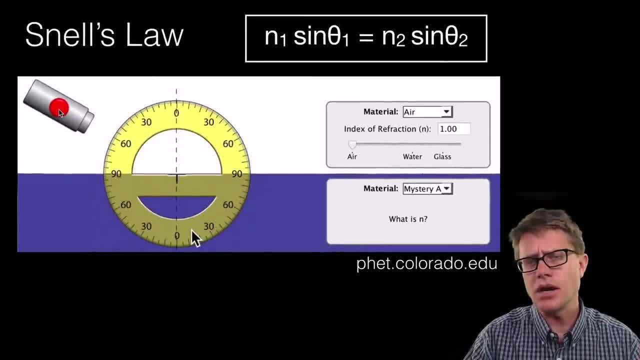 it is faster to an area where it is going to be slower. Now you could also have the problem presented like this. So, in this problem, what am I giving you? I am giving you the actual refraction. So it is coming in at an angle of 60 degrees. You can see that the 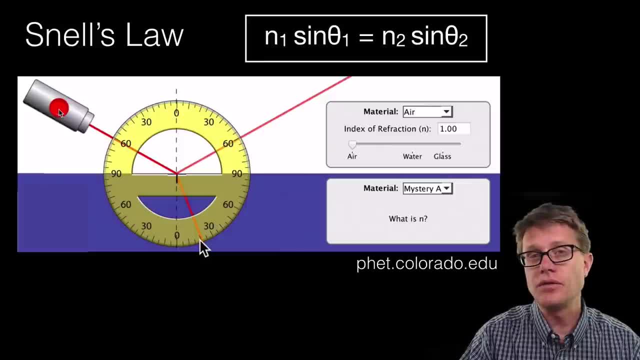 angle of refraction is going to be 20 degrees, And so could you figure out the index of refraction. Same thing: We are going to use Snell's law, And now you just have that one known, or those three knowns, and the one unknown that we do not have, It is going to be n2.. Now, what is? 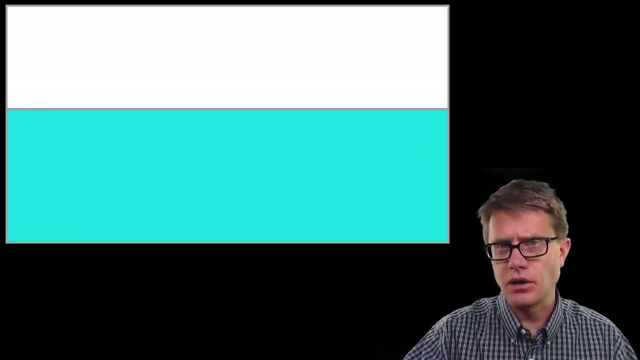 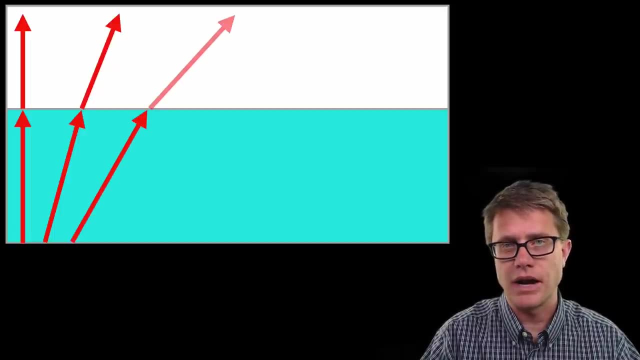 interesting is, if we look at material moving from an area of slow to fast, it would look like this: As we turn the angle, you can see that we are getting more refraction, But as we keep turning the angle more and more and more, you can see that less of that light is. 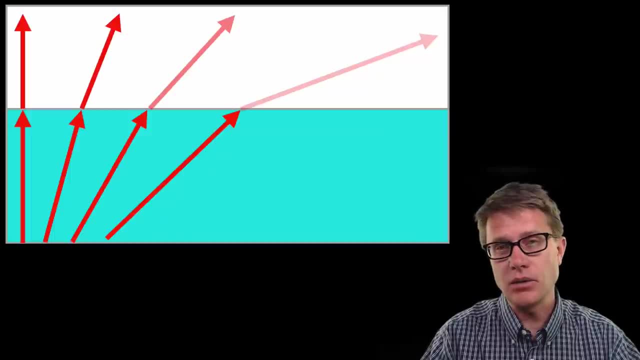 being refracted or making its way through, And eventually what we approach is something called the critical refraction. So let's do that. What we do is we take the angle of 0.577,, 0.577, and then we put in the deflection vector, And that is what we call the critical refraction. 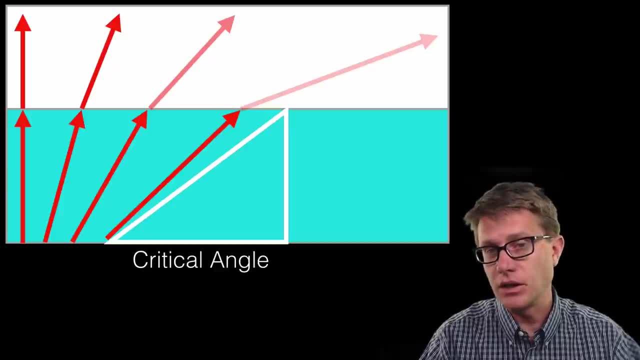 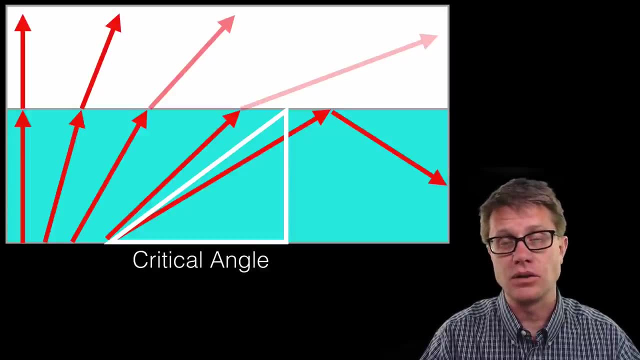 critical angle. Once we reach the critical angle, then we do not get light being transmitted into that next surface, And so what eventually happens is it is reflected back into this original medium. Now, when all of it gets returned back into the medium, we call that total internal. 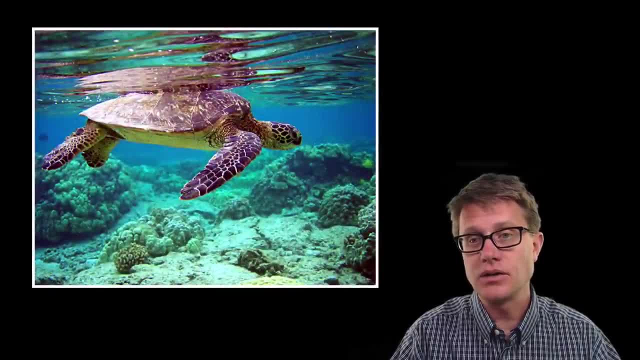 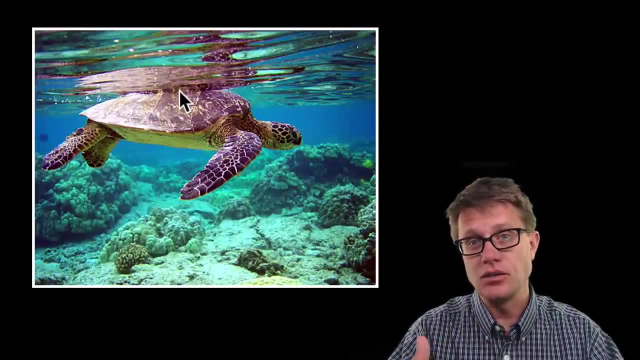 reflection. And so if we look at this sea turtle right here, the reason you are seeing its reflection up here on the surface is that light is not moving out. It is being reflected to you because of the angle at which you are looking at that turtle. And so did you describe.